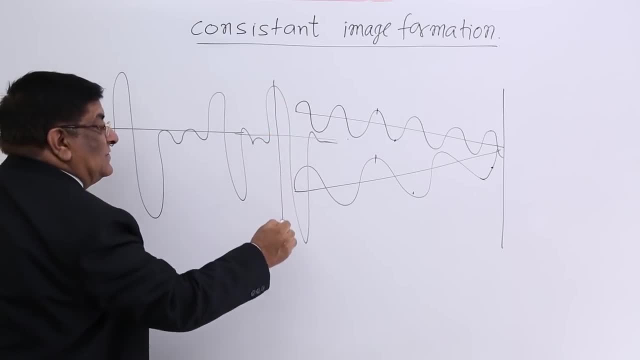 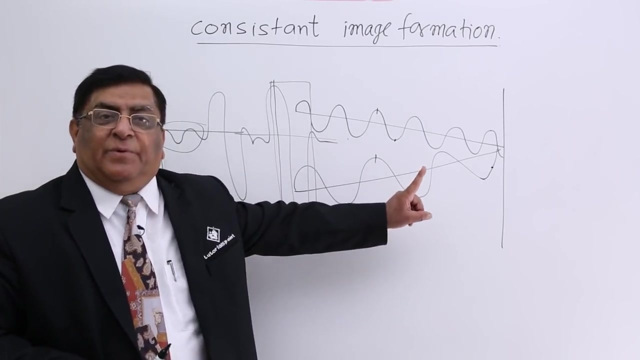 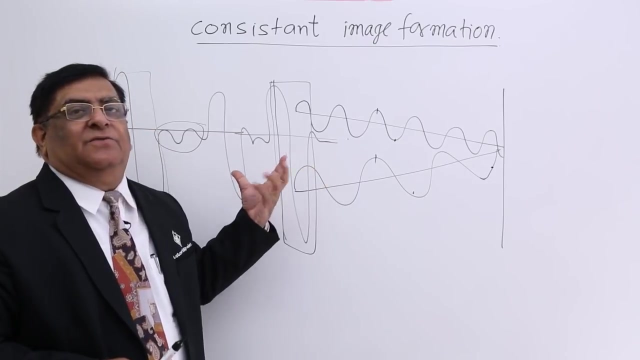 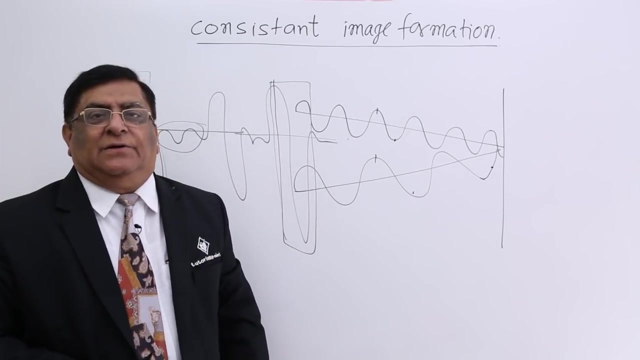 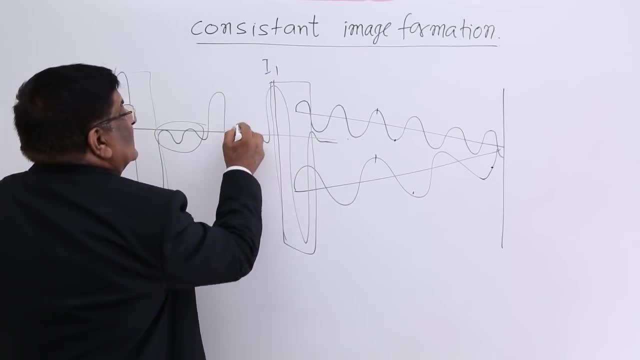 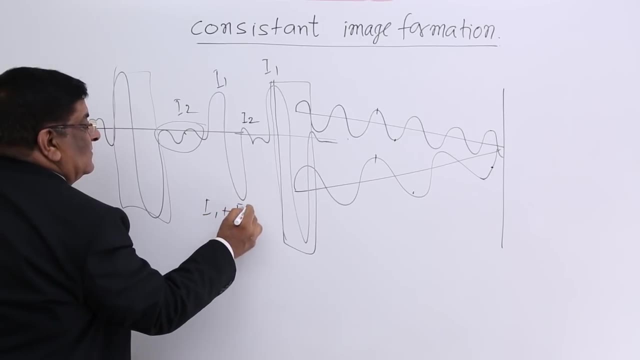 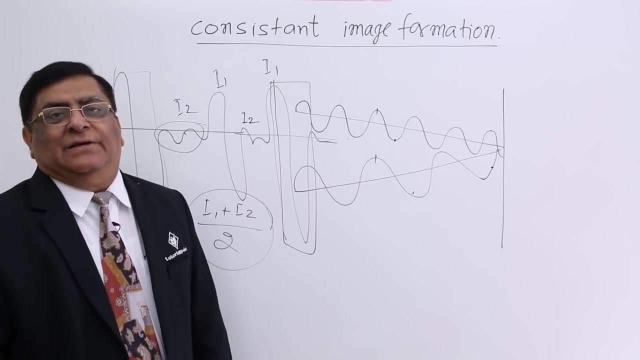 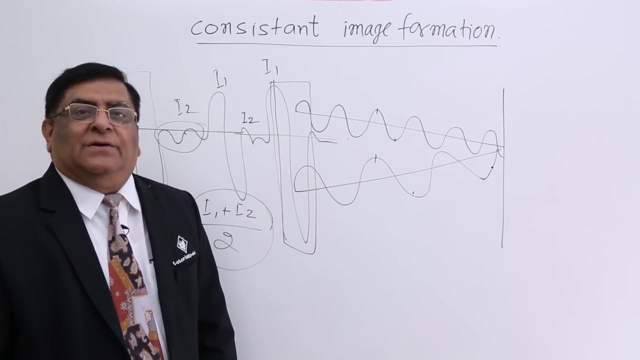 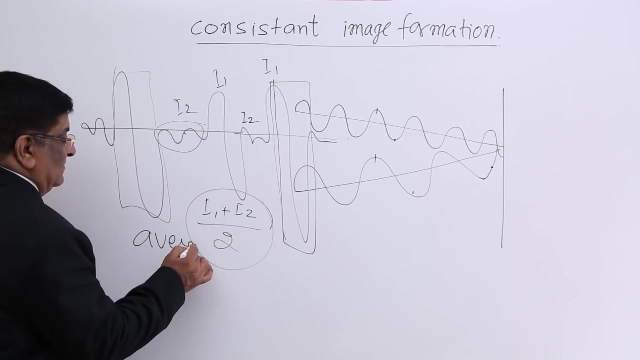 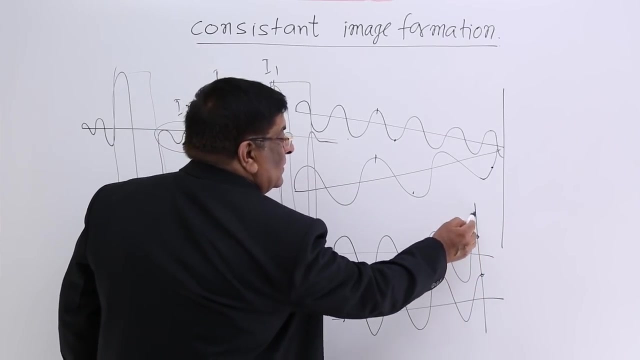 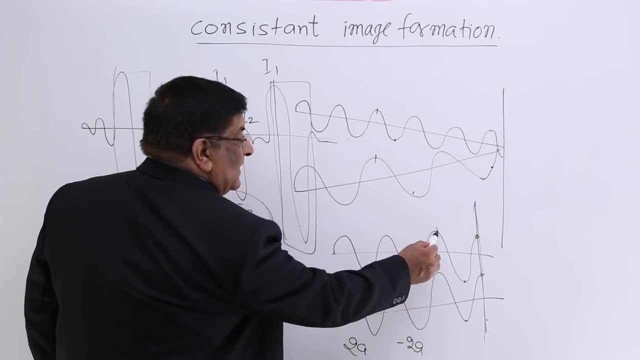 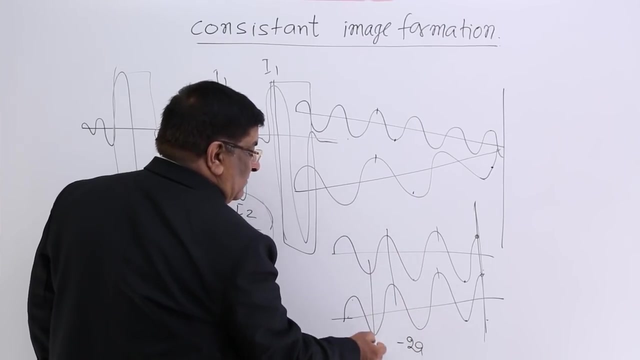 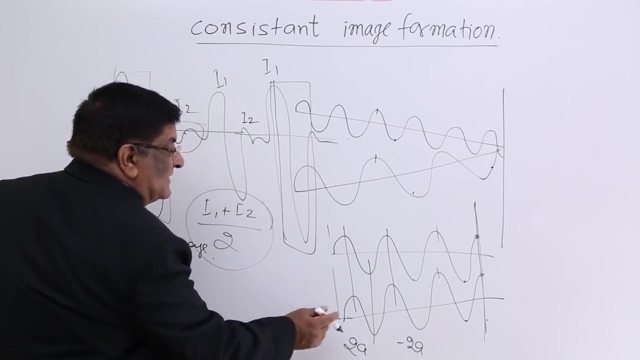 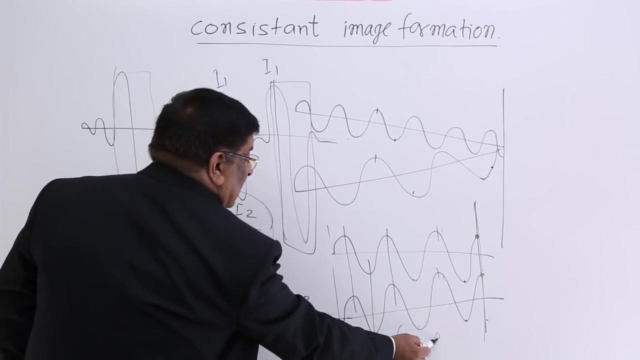 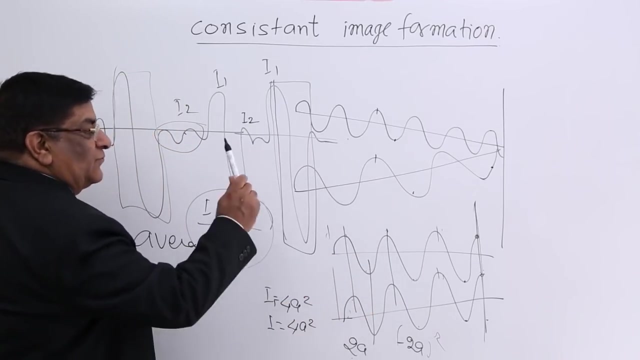 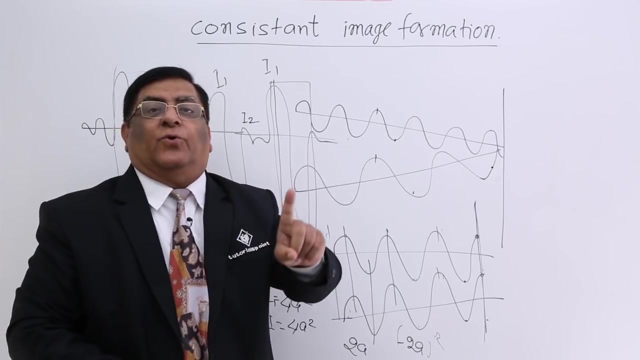 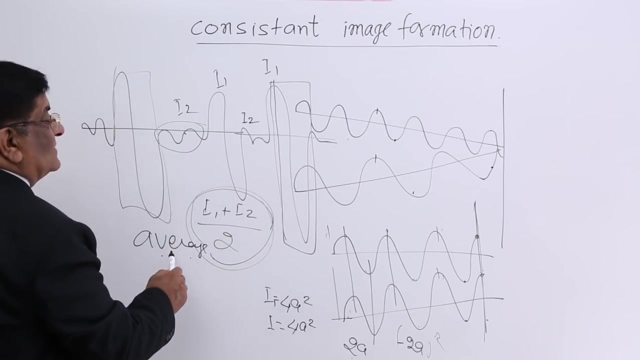 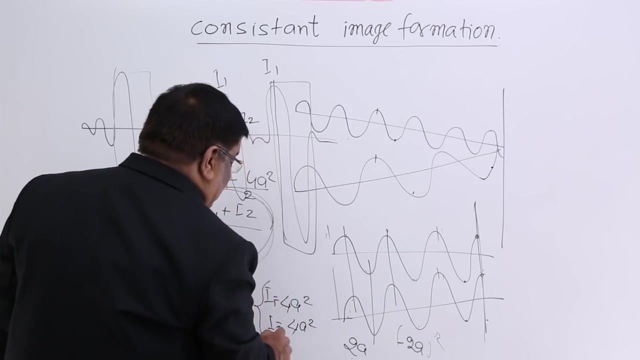 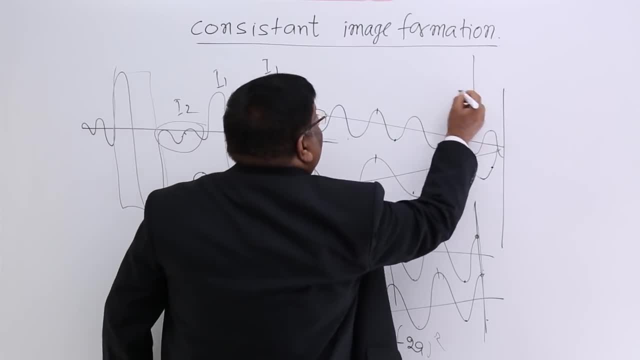 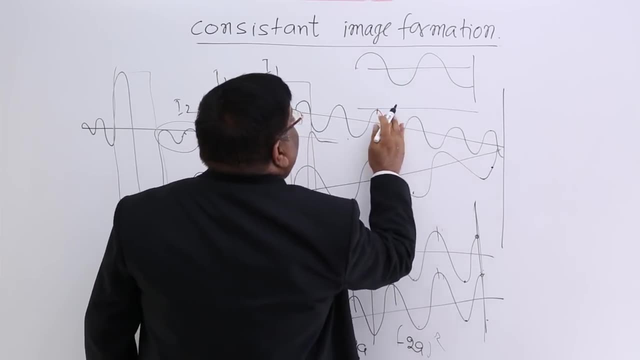 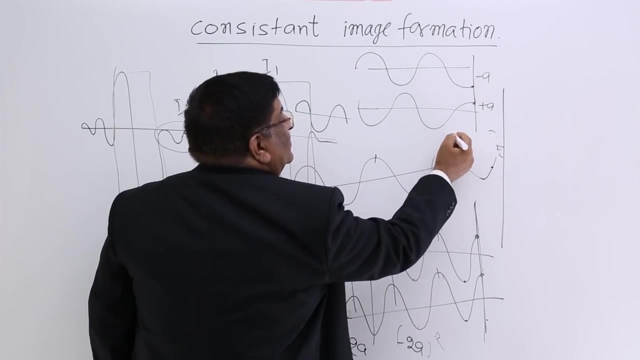 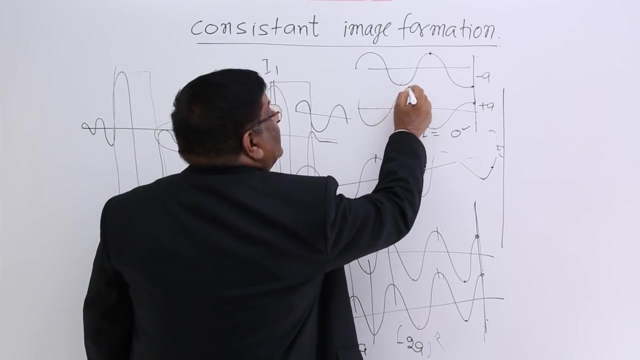 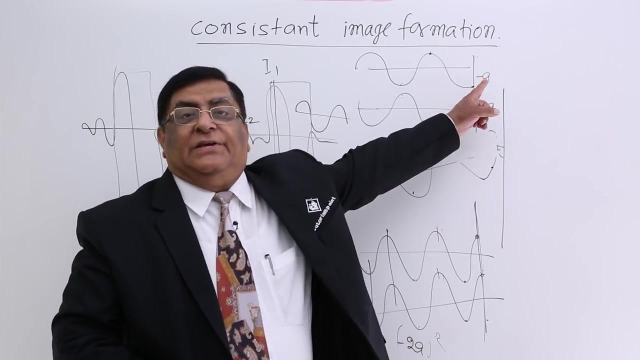 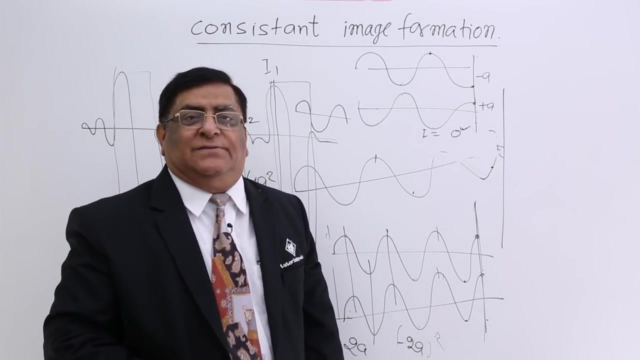 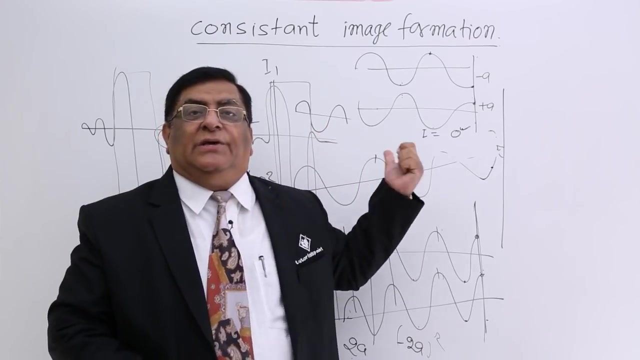 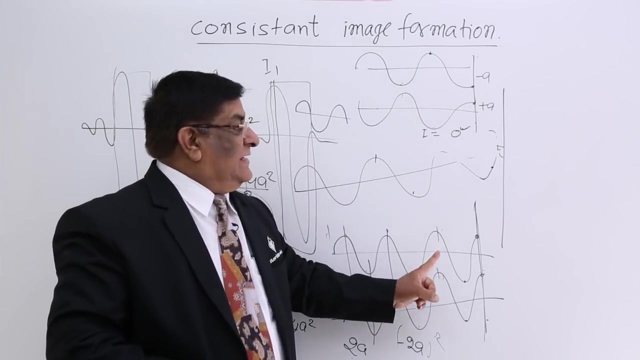 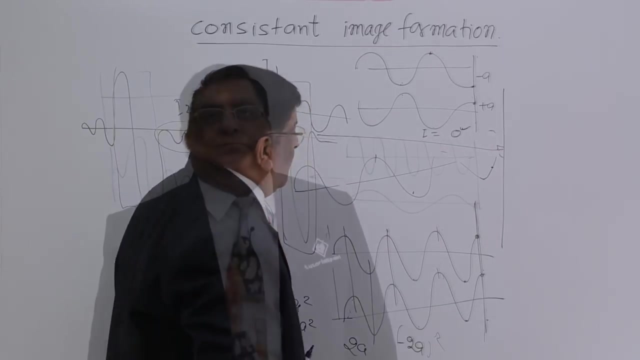 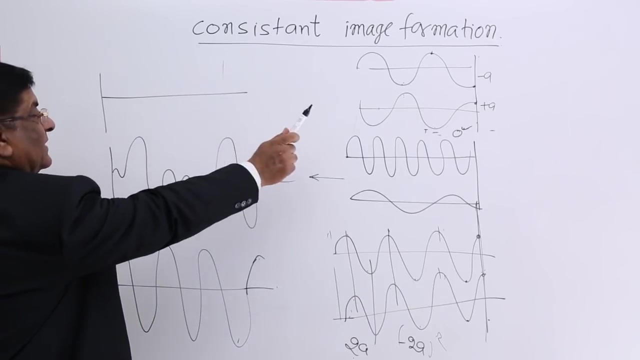 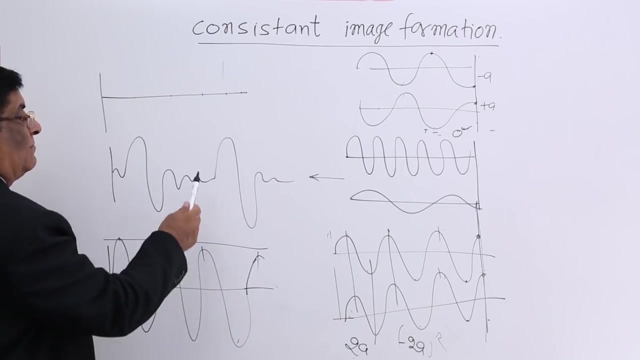 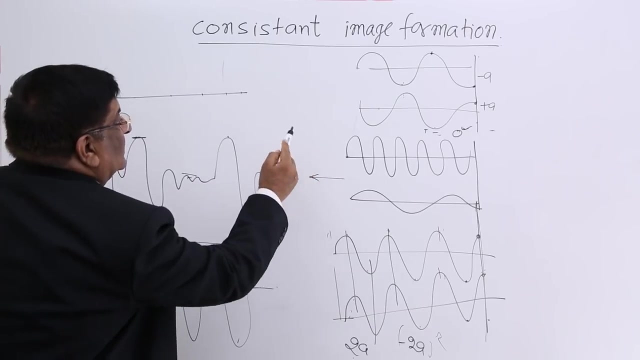 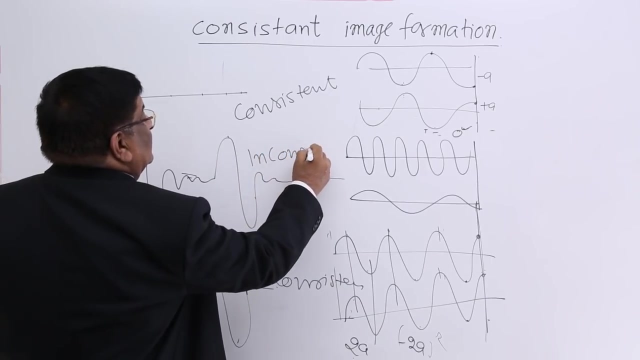 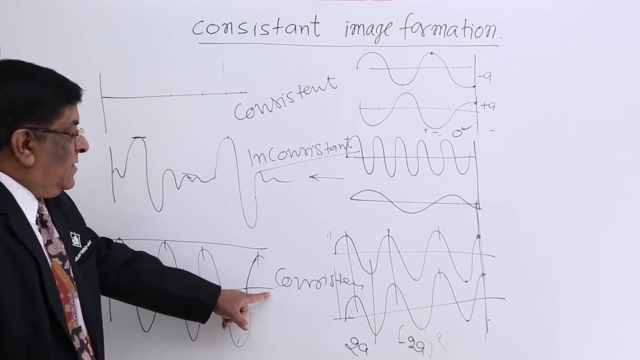 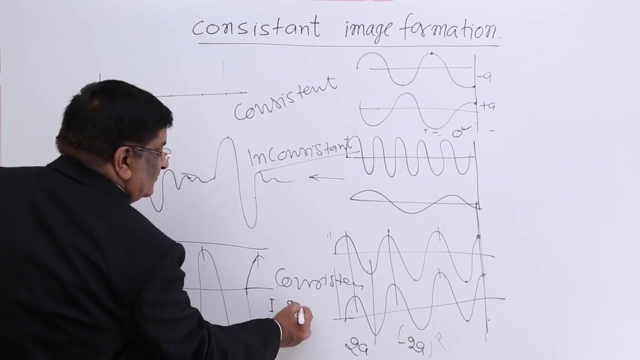 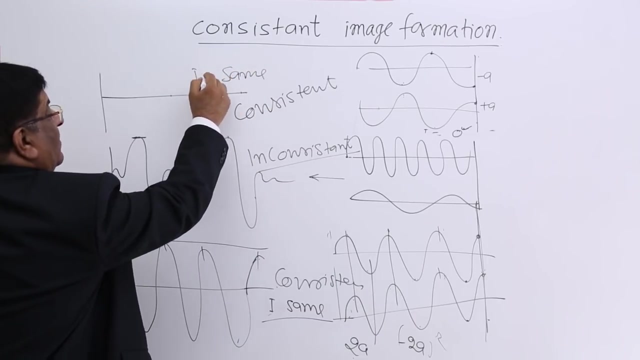 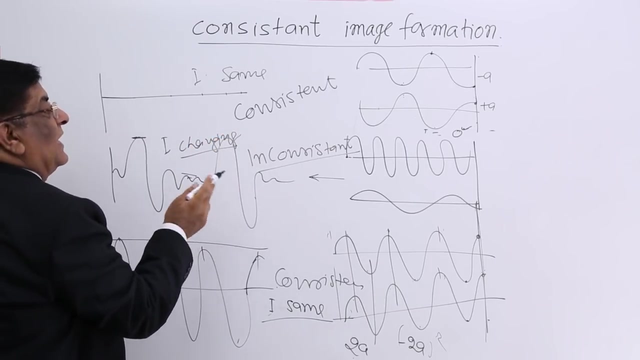 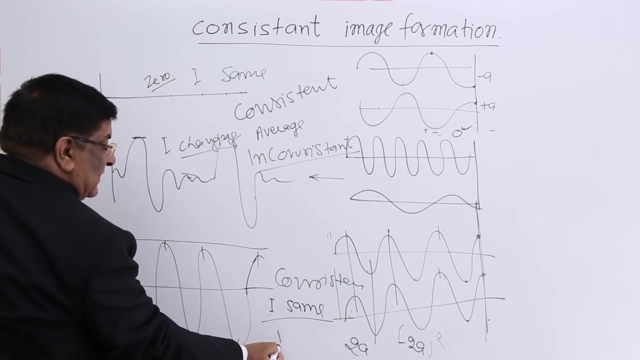 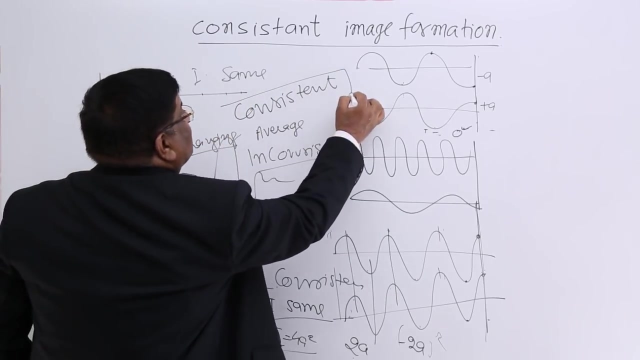 here. this is i maximum. so for seeing this effect or this effect continuously, what is required? the superposition should be consistent. then the image formation will be either bright, 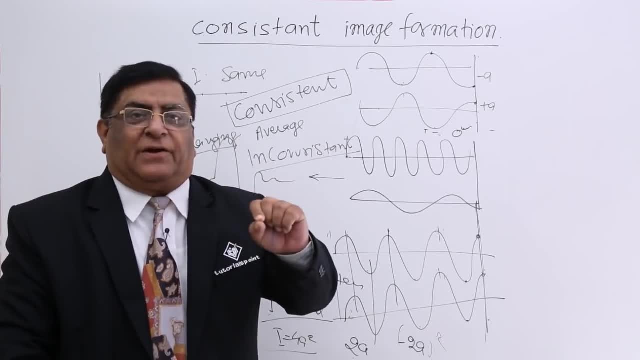 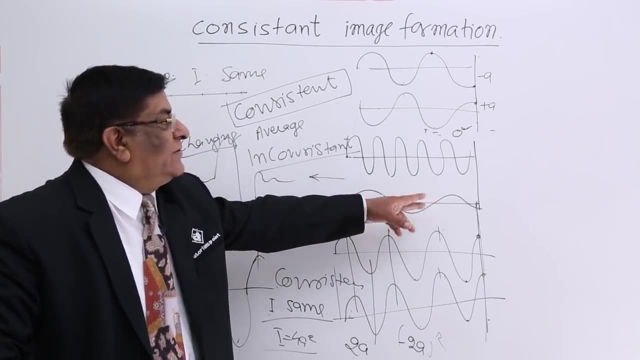 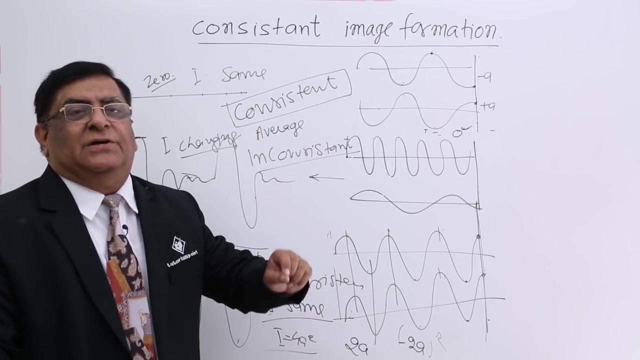 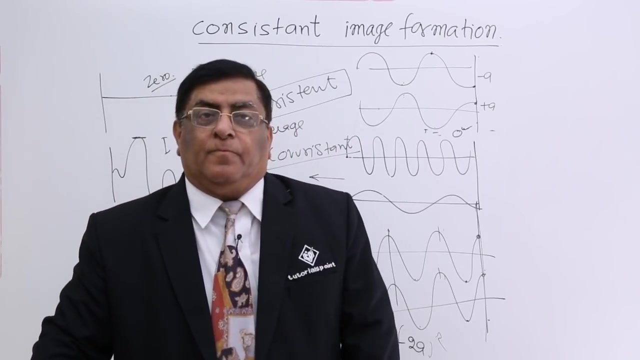 or dark, and we will be able to see the effect of superposition. and if they are like this, sometimes crest on crest, sometimes crest on trough, we will not be able to see the effect of superposition, constructive or destructive. what we will see is a average light. now, if